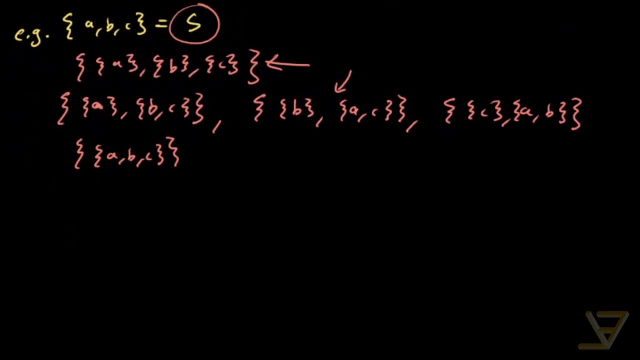 What we are going to be looking at are K partitions. K partition is a partition containing K sets, So this one here is a three partition. This one, this one and this one are two partitions And this one is a one partition. 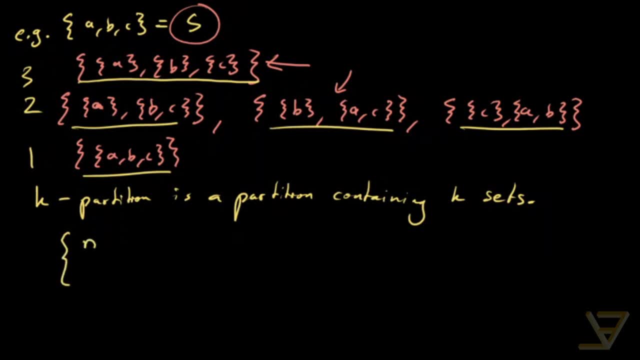 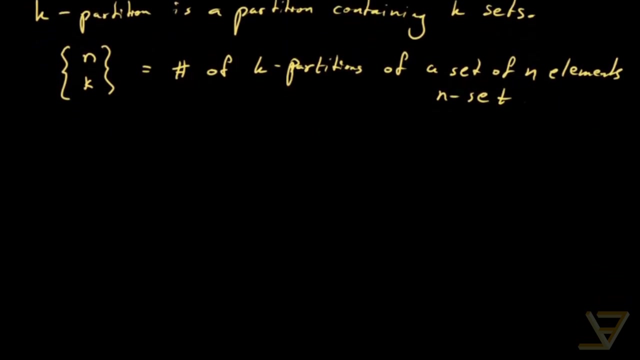 We're going to denote by N split K. That's what I call this. I don't think it's standard. N split K is number of K partitions of a set of N elements, otherwise known as an N set. So let's do a couple of computations. I'm not going to show exactly how these are done because I'll give a more general formula at the end. 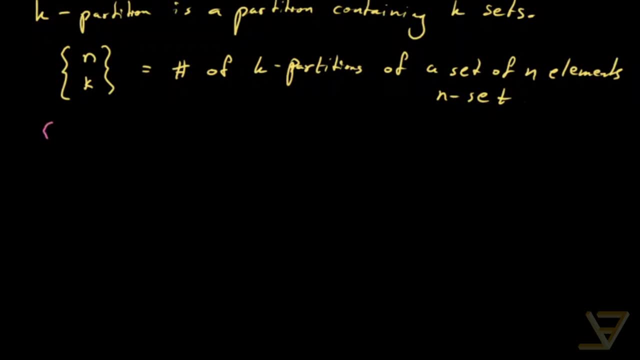 But a couple of computations. four computations that I'll show you are: N split one can be done in exactly one way. N split N can be done in exactly one way as well. N split two can be done in two, to the power of N minus one, minus one ways. 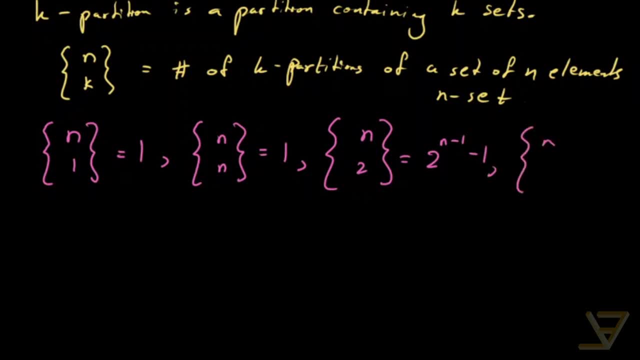 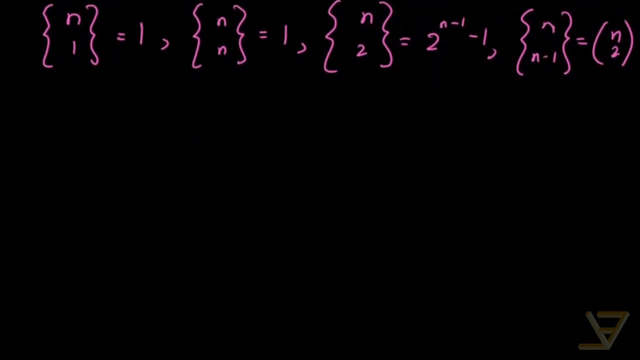 And N split N minus one can be done in N choose two ways. These are fairly standard identities and you can look them up in many places, including Wikipedia. So what we want is a general formula for N split K, And it's not going to be a pretty formula, but it is going to be a formula that we can use for computations. 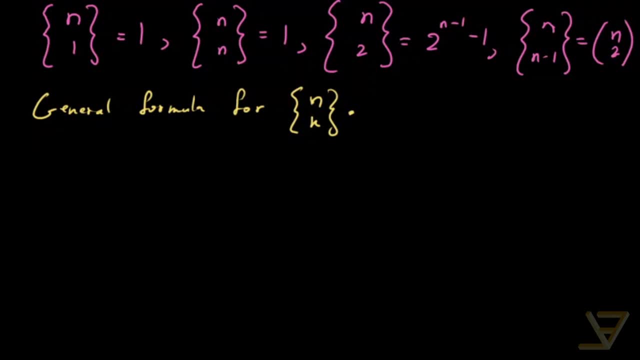 What we have to notice is that the number of ways of splitting, let's say the first N positive integers, one, two through N, into K non empty sets, is the same as the following: Distributing N distinguishable sets. So these are the N distinguishable balls that we have.